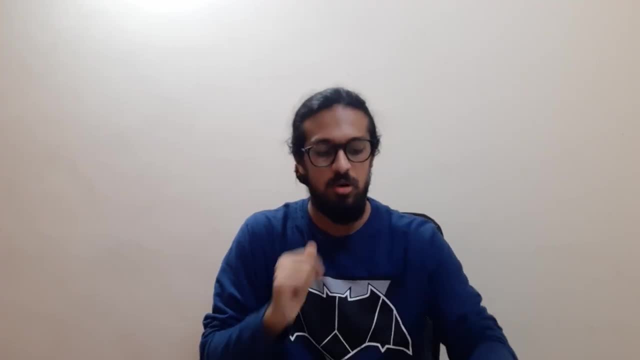 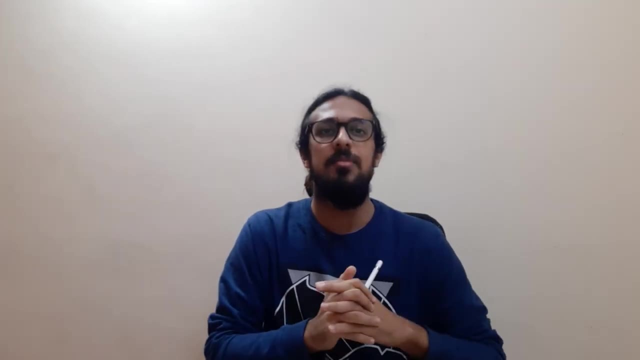 In today's video we'll be talking about the SIS model, which is a popular model used in disease dynamics. The scope of today's video will mainly be describing the SIS model, finding the equilibrium points of the SIS model, finding their stability. 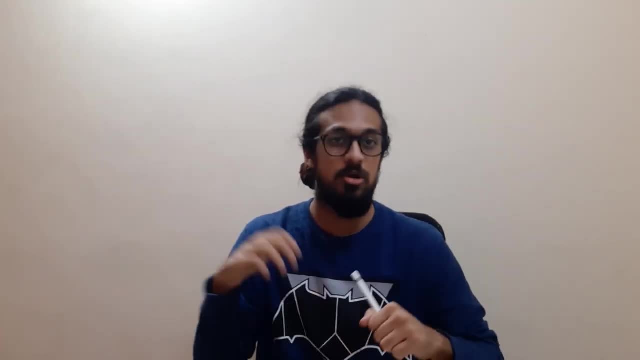 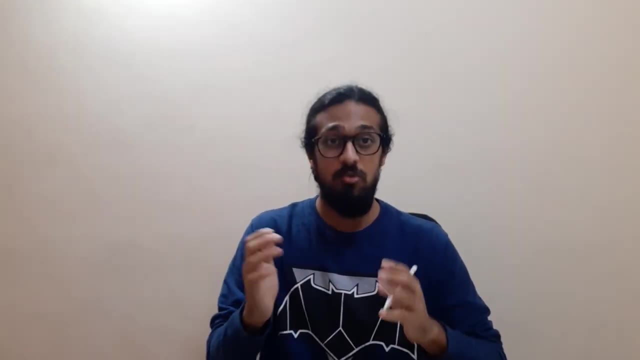 and also a little bit about the solution curves and reproduction number. While I do mainly focus on only the disease dynamics aspects of the SIS model, this model can also be used in other fields and other applications where you have a similar kind of flow of population, as I will soon explain. 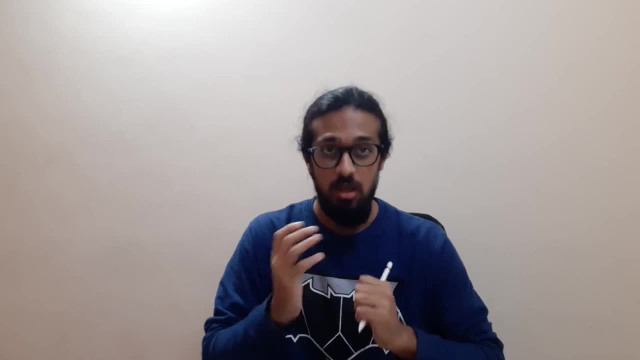 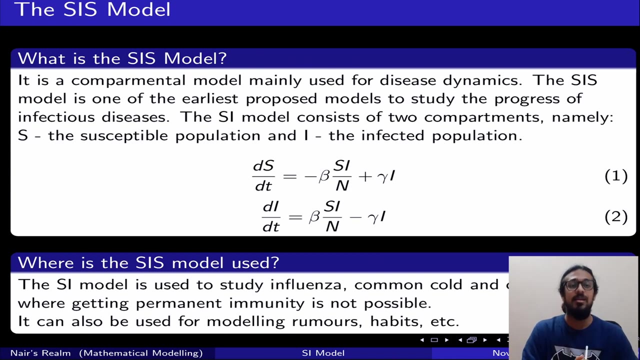 So, without further ado, let's get started with the SIS model. So what is the SIS model? The SIS model is a compartmental model, And if you're not sure what compartmental models are, I've already explained it in. 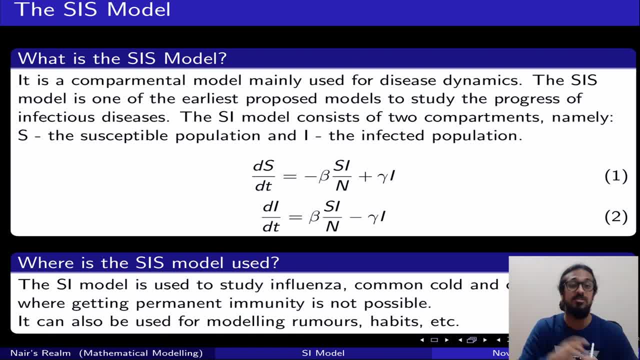 my mathematical modeling video, which I'll link right here and also in the description so that you can check out. It was one of the earliest suggested models to study disease dynamics And there is a slight difference between the SI and the SIS model. So some 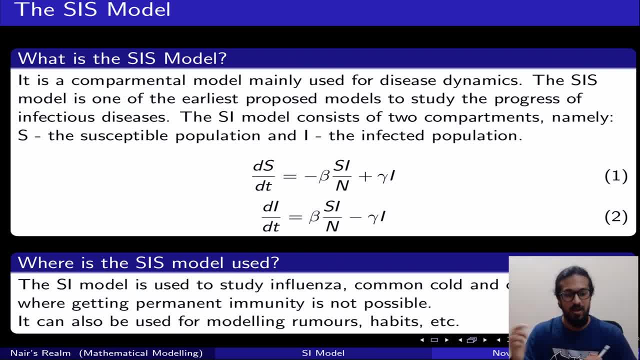 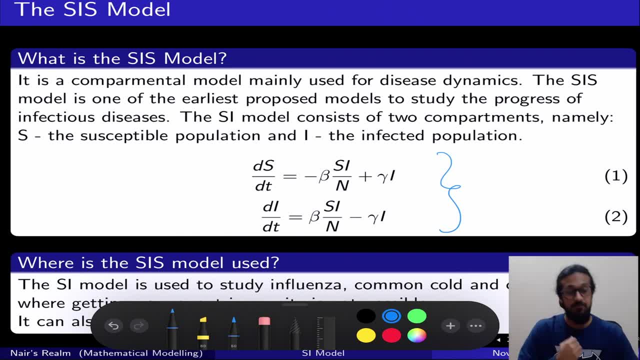 of you might be aware of the SI model and you might be thinking: why is it different from what I've put down here? So I will try to explain what the difference is through an example. So let's take the HIV virus. All of us are susceptible. Everyone in the entire world is. 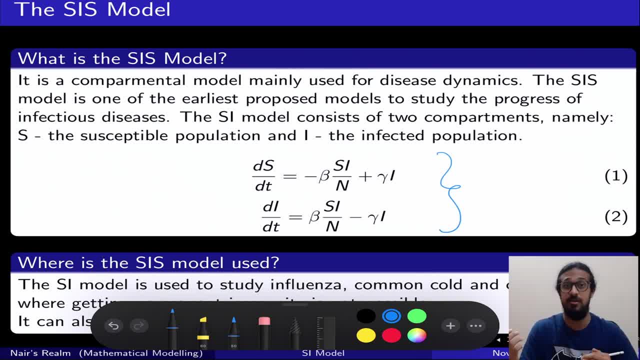 susceptible to getting the HIV virus and there is no cure for it today- And therefore, if you do get the HIV virus, you will stay infected. So if you were to look at this and try to figure out the flow of the populations, you would see. 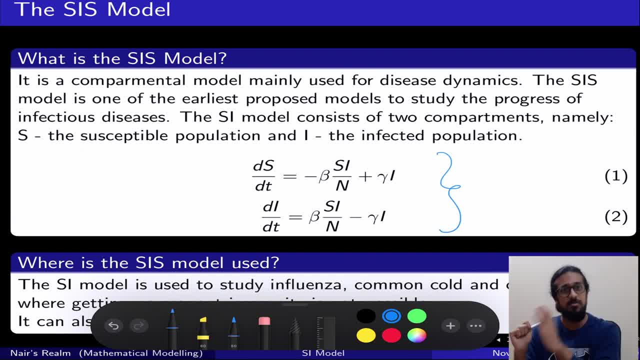 that everyone is first in the susceptible population. Some of those individuals who get infected move to the infected population. That is the only flow. Once you're infected, you stay infected until death and there is nothing else that can flow either way. So that is the strict SI model, where there is a flow only from the S compartment to the I compartment. 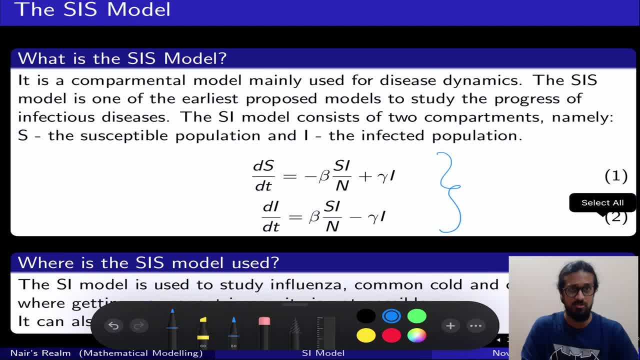 Now, if I were to talk about the SIS model, which is the scope of today's video, I will explain it again with another example. Take the common cold. Many of you might have gotten the common cold in 2019 or 2020.. Now that means you are susceptible and you got infected. 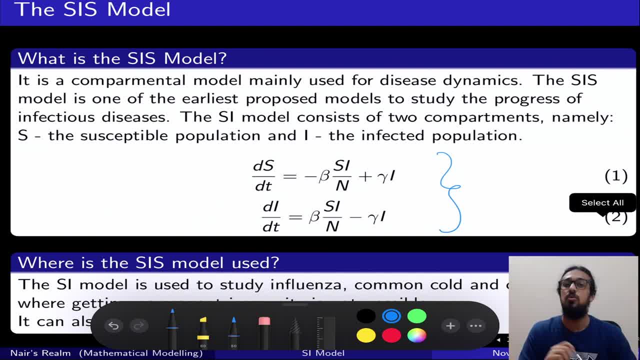 with the common cold, You took a few pills or took rest, as per your doctor's suggestion, and you recovered from it. Now, in this case A, you can recover from it. B, however, you don't have permanent immunity or long-lasting immunity. What I mean by that is: so you got it in 2020.. Now it's 2021,. 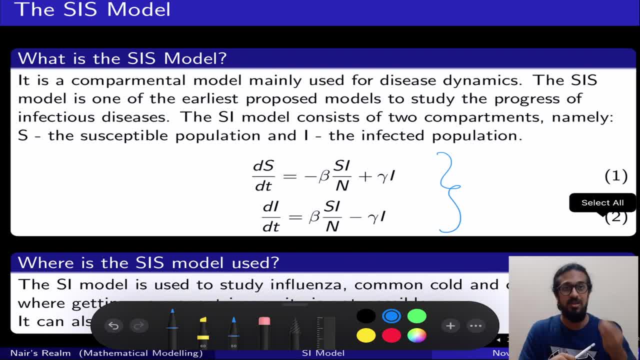 it's flu season again. You are again a susceptible individual to that disease. So that is the SIS model. Why, If you think about the flow, you were susceptible, you got infected And once you recover you go back to the susceptible population. 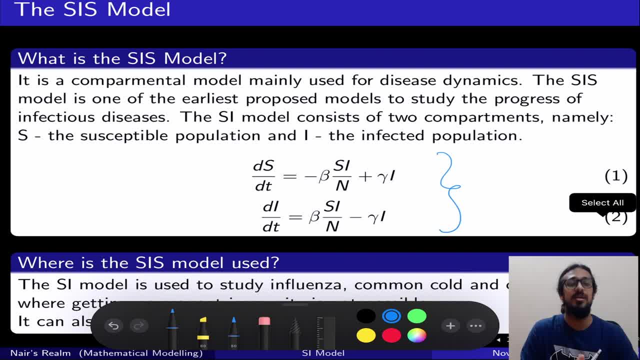 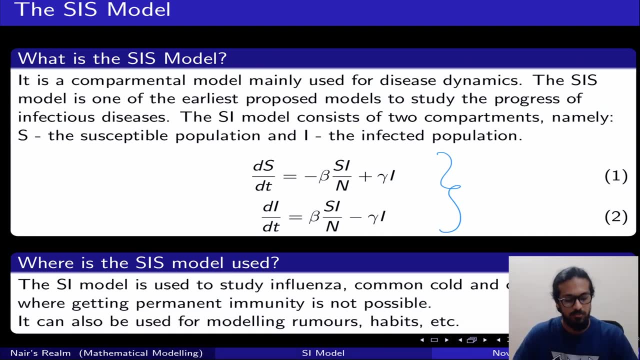 Which essentially means that the SIS model is suitable for those diseases where reinfection is a common occurrence or reinfection can happen very easily. So let's take a look at the differential equations that describe the SIS model, And I do hope the difference between the SI and the SIS model are clear. 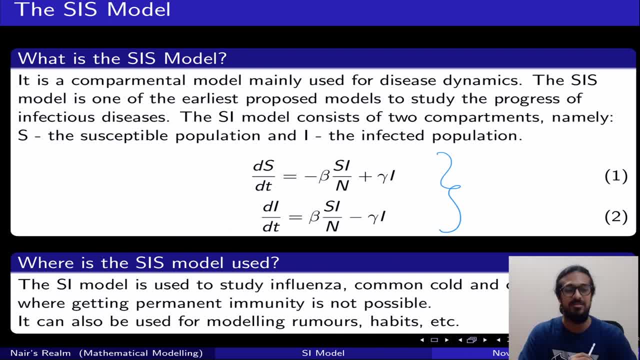 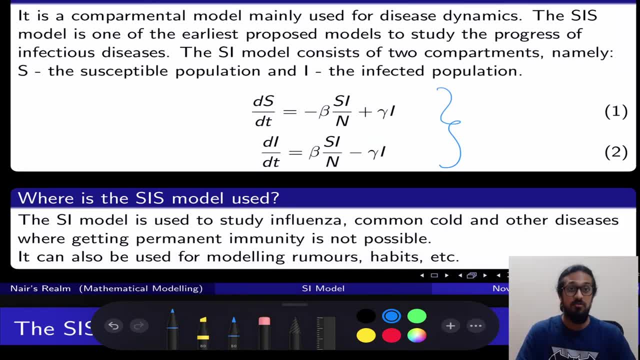 If not, make sure you drop a comment and I'll try to address it the best way I can. So the SI model Essentially has two differential equations which govern its dynamics. There is one for the S compartment, which is the susceptible population, or all. 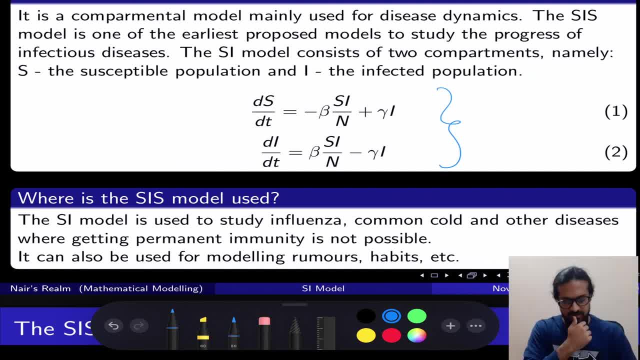 those people who are susceptible to getting the disease. And there is another differential equation for the I population, which is the people who are already infected. Now I will explain a bit more about it in the coming slide, but I just want to mention that the SIS model is mainly used in disease dynamics. 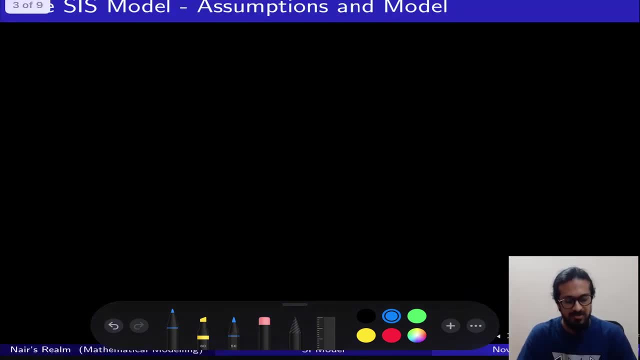 but again, like I mentioned, can be used in other places as well. So let's get started with the SIS model. So this is the SIS model. We have two differential equations here. So now, if I were to explain in terms of compartments, 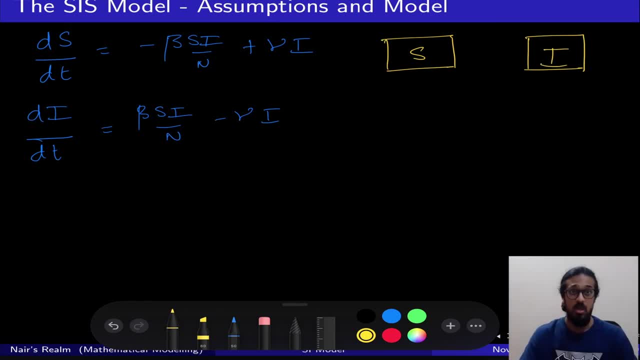 I have an S compartment and I have an I compartment. right Now. everyone is susceptible. Now, once they do get the disease, they leave the S compartment and go to the I compartment. So I would represent it this way: that there is some outflow from the S compartment. 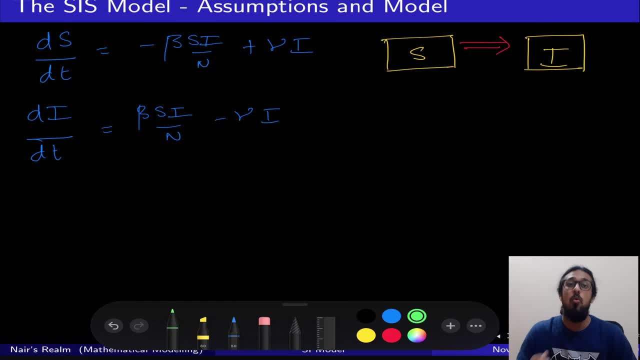 And once you do recover again, you are susceptible. So there is some inflow to the S compartment Now. the red and the blue are the outflow. So the red and the blue are the outflow Now. the green arrow which I've drawn actually is the beta SI by N term. 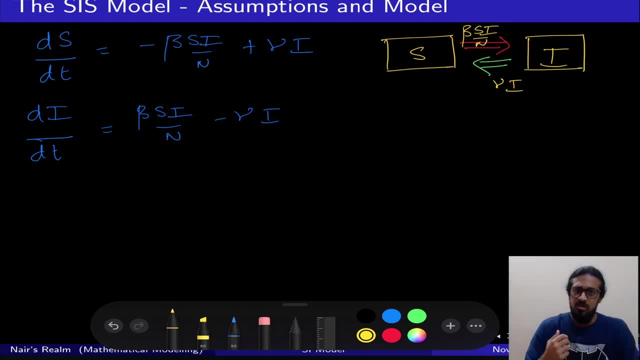 and the green arrow is actually the gamma I term. So there are a couple of questions, obviously, which you will have: what is beta and what is gamma? Before I get into that, I just want to speak about one particular assumption which has been made in this model. 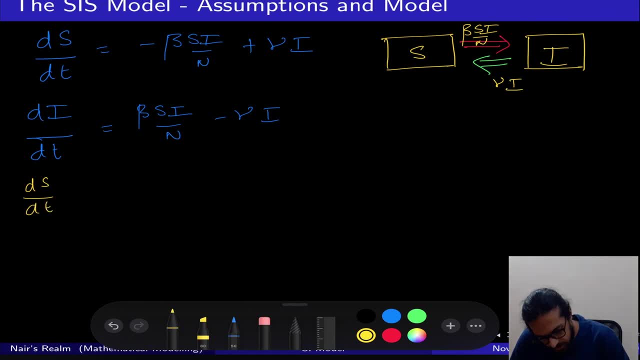 So if you want to do dS by dt plus di by dt right, which is dS by dt plus dI by dt right, by dt, into s i, from the above two equations we can see that you will actually get zero. so what do i mean by that right? so what i mean by that is that the total population. so 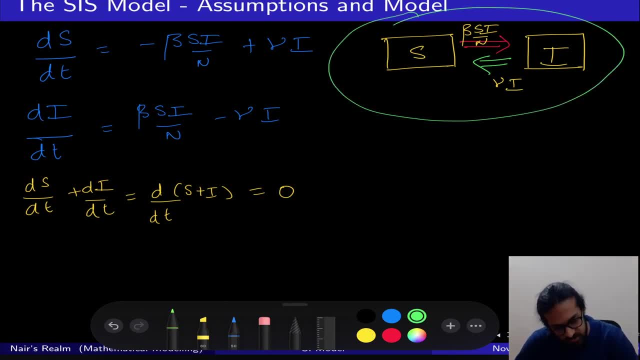 if i were to explain to you this way, this is our total population. let's call it n. the only two compartments like i was talking about is the s and the i compartment. so you either go from s to i and then back from i to s, but that is the only flow which these diseases take. so 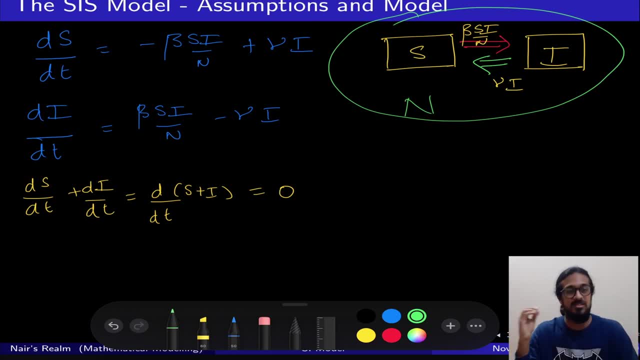 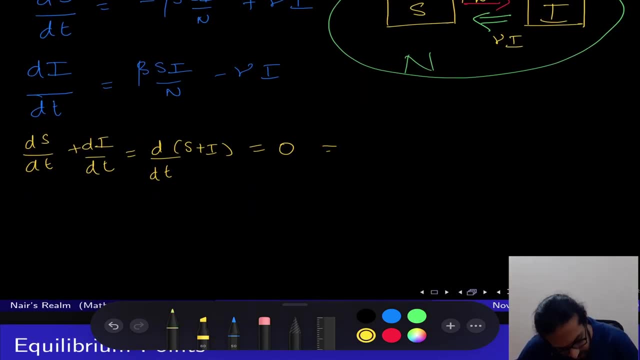 the entire population was essentially nothing but the sum of the susceptible and the infected population at any instant of time. so this, so this implies that dn by dt is equal to zero, which essentially means that the rate of change of population is zero, or which implies that the 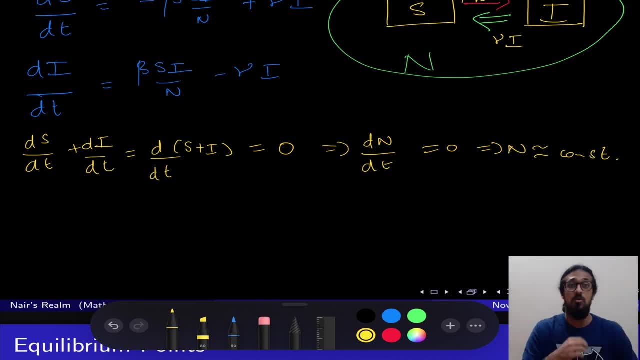 population is constant. now, is this assumption correct in the first place, or when can we make this assumption so the population can be constant if the natural birth and death rate in that region is somewhat similar? a good example for that in today's world is germany, where the natural birth rate and death 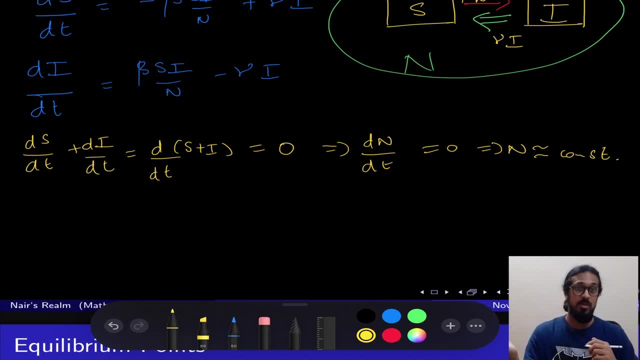 rate are fairly similar. it may not be accurate in a country like india, where the birth rate is much smaller. so this is a very simple assumption. but you can think of it this way: that if you're modeling something over a short span of time- let's say a month or a couple of months, and you're dealing 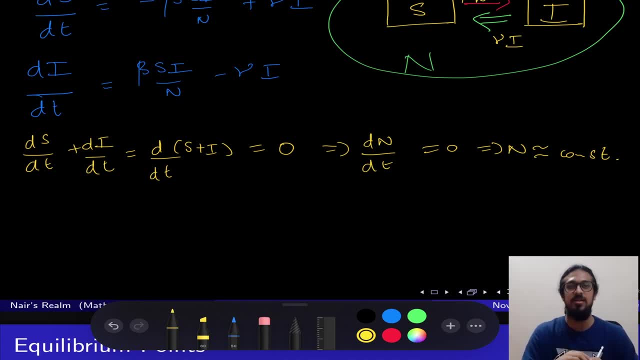 with a disease where the mortality rate is close to zero, right. so so if someone gets infected with that disease, they're not going to die, they may just transmit that disease to other people. so trying to study some disease like that over a short period, then it's fair to assume that the 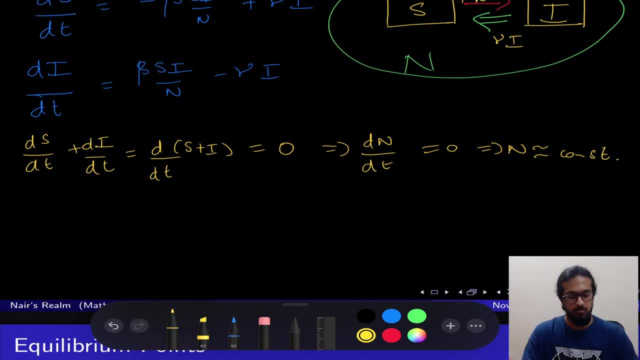 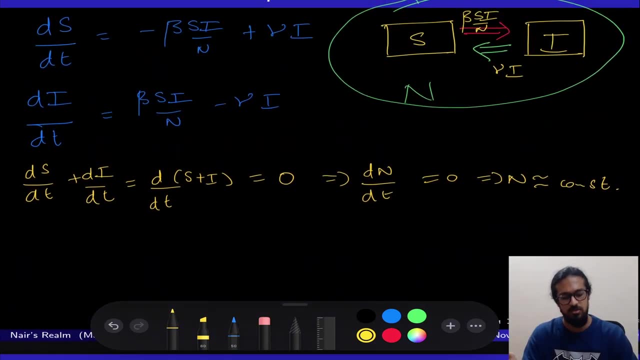 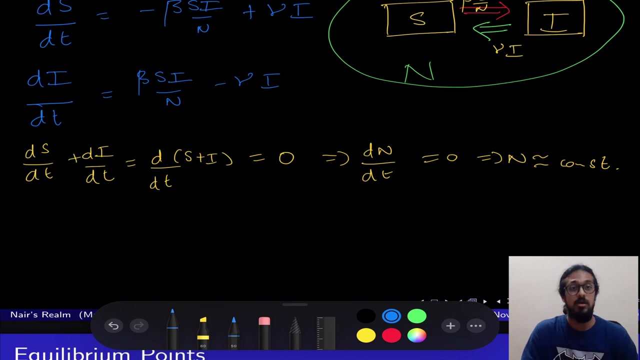 population will more or less be a constant. talking about the non-constant SIS model as well in a subsequent video, But for the scope of this video, we are dealing with this model where the population is constant. Okay, so now that we are. 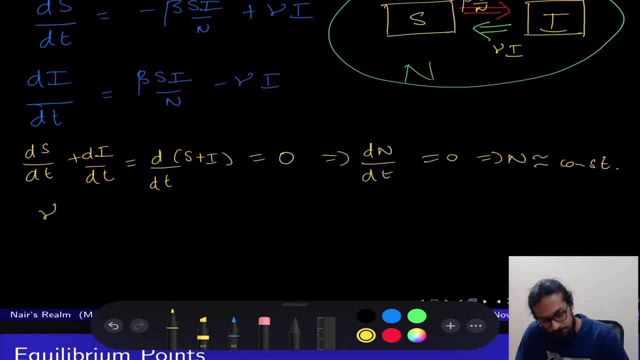 clear. on the assumption, let us talk about the two terms beta and gamma. What are they right? So in mathematical modeling of diseases, beta is commonly described as the transmission rate, or in other words, it's the rate at which the disease is transmitting. Now it is a variable. 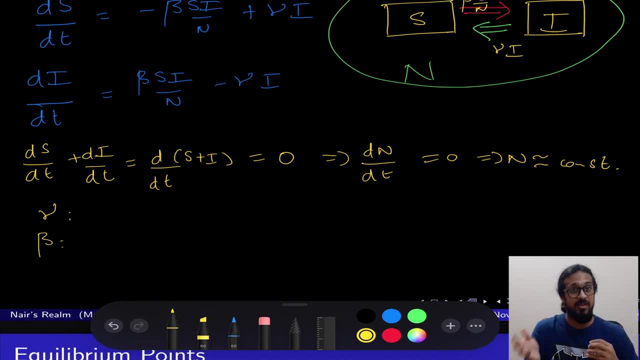 value and it varies from disease to disease. It can also vary within the lifespan of a disease and a good example for that is the coronavirus right? So when the coronavirus started we had the initial strain and the the. it was infectious and it spread rapidly around the world. But when the Delta variant came about, 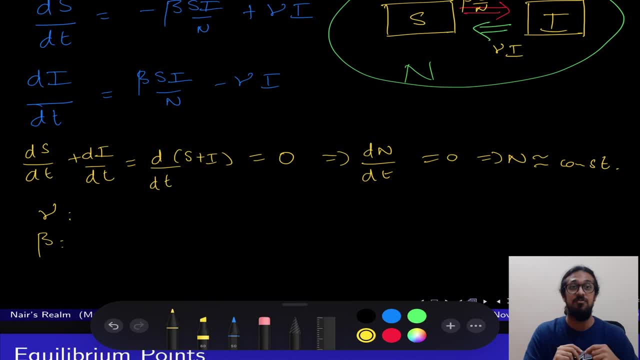 we got to know that the Delta variant is much more infectious. Therefore, the transmission rate of the Delta variant is much higher than the initial strain. So you can see how the transmission rate can be a time varying parameter. But for known diseases which have existed for a very long time, 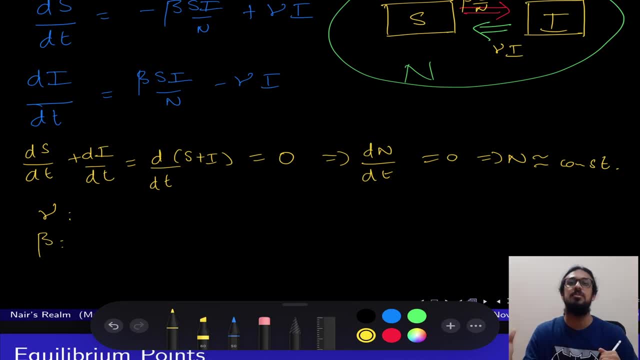 there are studies which have been done to give us a fairly good estimation of the value of beta. So beta is the transmission rate. What is gamma? Gamma is the rate at which an individual recovers right. So you get infected with the common cold, you take rest, you eat a few medicines for a week and then you're fine. 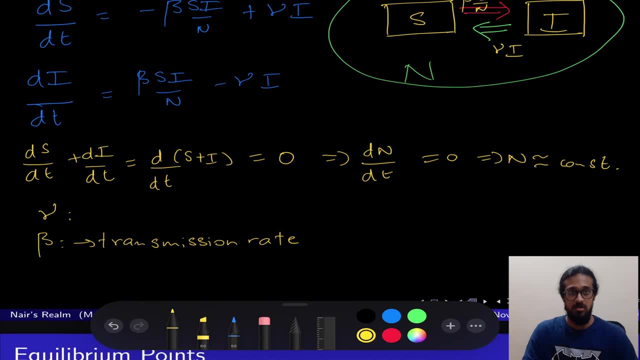 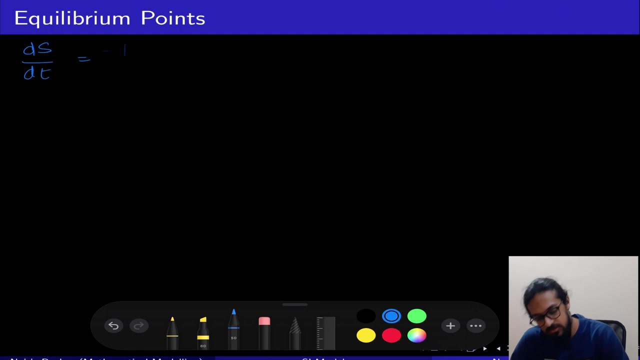 So the rate at which you recover from a particular disease would be the recovery rate, and that is the term gamma. OK, so, as you can see, there are some 감� bests or there are some teaspoons, to be sure, that's not크. 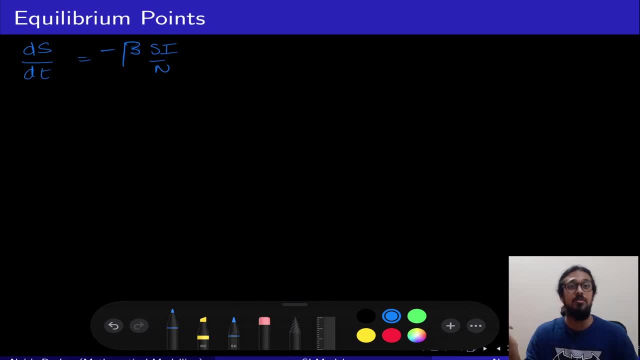 Initiatives. It doesn't count up, right. So these just includes times and units, only you times And all the other sufetias, All right. So now that the assumptions and the model is fairly clear, let's move ahead to the next aspect of any dynamical system, which is the equilibrium points. 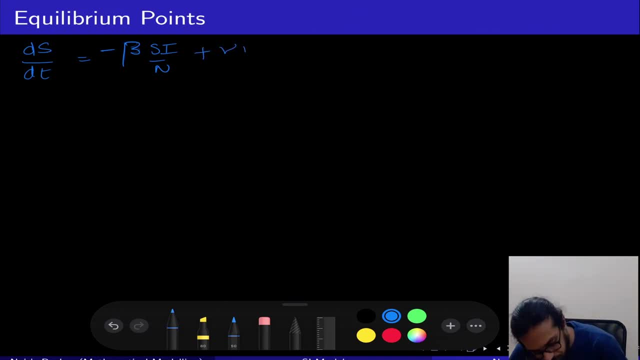 link to the video here. you guys can check it out, so i'll just write the model here. equilibrium points are also called fixed points, and what we mean by that is at those particular points the state of our dynamical system is fixed. so what do we mean by that? we essentially mean that the 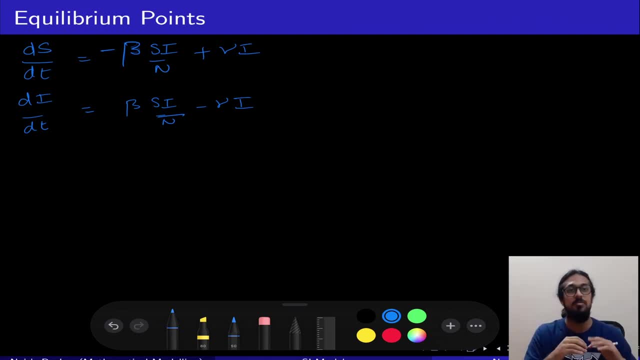 rate of change of the dynamical system as a whole will be zero. so the dynamical system is in a constant state. now the way to find equilibrium points is to equate, uh, both the ds by dt term to zero and the di by dt term to zero. because when all the state variables involved, in our case the 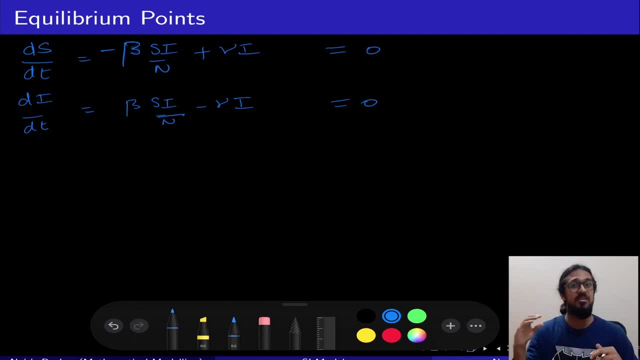 state variables are i and s. when all the state variables involved have a rate of change as zero, which means they're all constant, we are in an equilibrium state. so now, if we were to solve these two simultaneous equations we can see from, you can take any one, so i'm going to take the first. 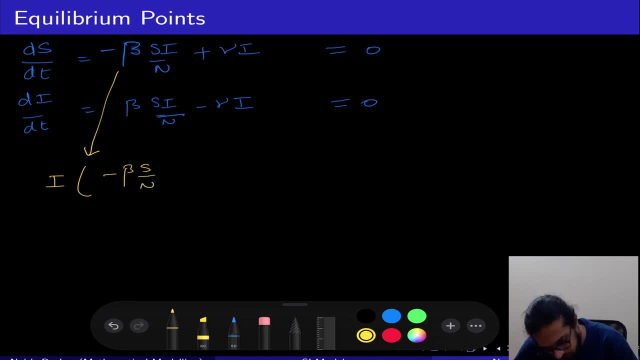 equation and i can see that now, if i equal to zero, we can see that this satisfies, and for any value of- sorry about that- for all- s this equation is, both these simultaneous equations are satisfied. however, if i is not equal to zero, then what happens? right? so then we see that s is equal to. 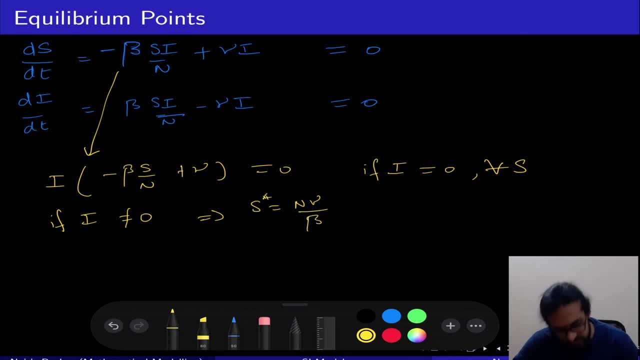 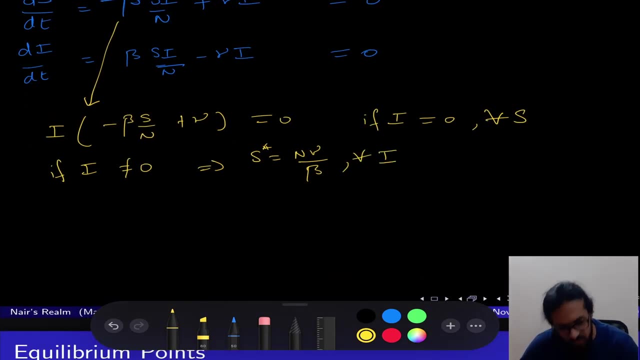 n times gamma by beta. this is the equilibrium point and this will be satisfied for for for any i. so you can see we have two sets of equilibrium points here. one is any s comma zero and we have n comma gamma by beta, comma any i. okay, now that we have solved. 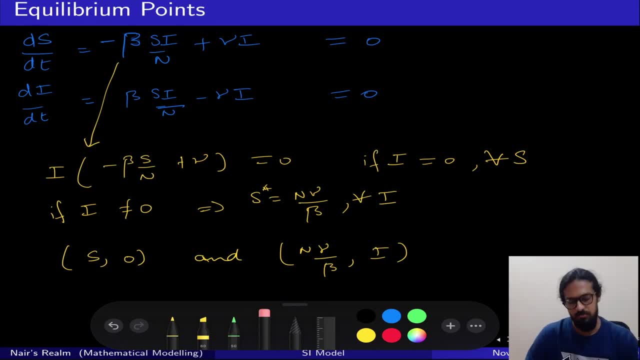 for the equilibrium points, we can see that there are two sets of equilibrium points. one is s comma zero and the other set is n times gamma by beta comma i. now, while there are an infinite number of equilibrium points in disease dynamics and mathematical modeling of diseases, we mainly are: 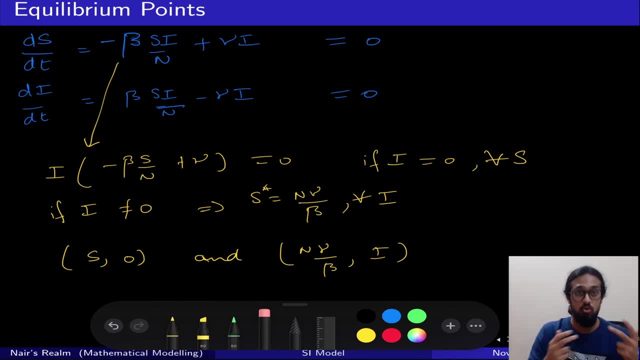 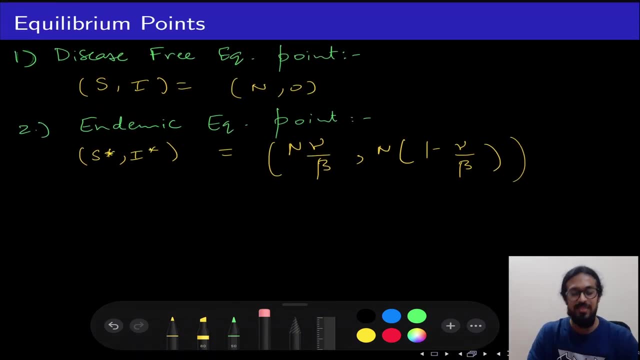 interested with two sets or two specific equilibrium points, so to speak, and those are the disease free equilibrium point and the endemic equilibrium point. now, the disease free equilibrium point is that state where nobody is infected, or everyone is free of the disease, right? so that essentially means that the 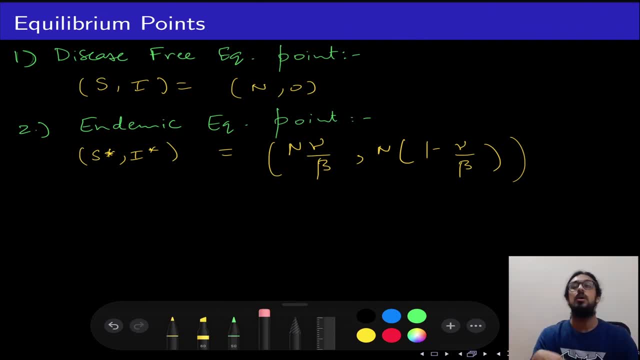 entire population is just susceptible. so that could be thought of as the starting point of any disease. now the endemic equilibrium point is actually much further along into the disease, once the disease has progressed and has reached kind of a steady state or an endemic state. in technical terms endemic refers to a localized 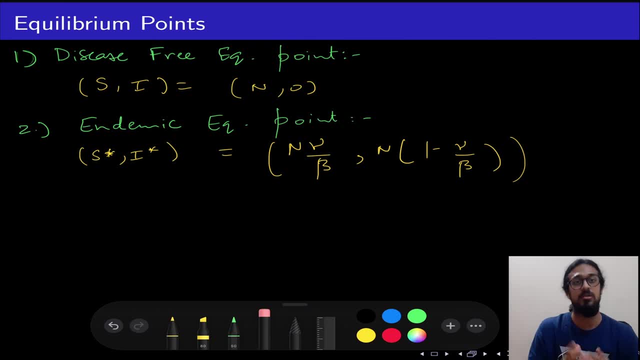 disease pattern. so, for example, in the case of coronavirus, it was viewable and if it were to reach endemic state within each country as well, we would see outbreaks in small regions of each country. that would be an endemic state and therefore it makes sense to discuss stability. 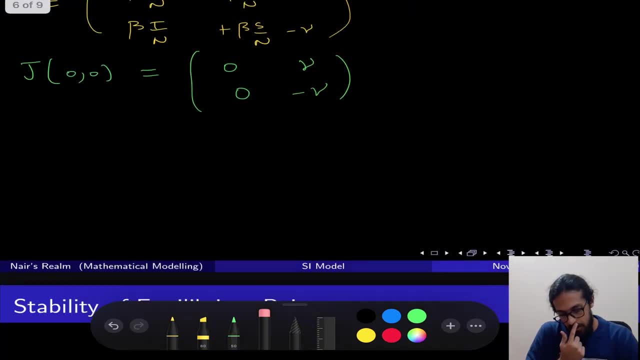 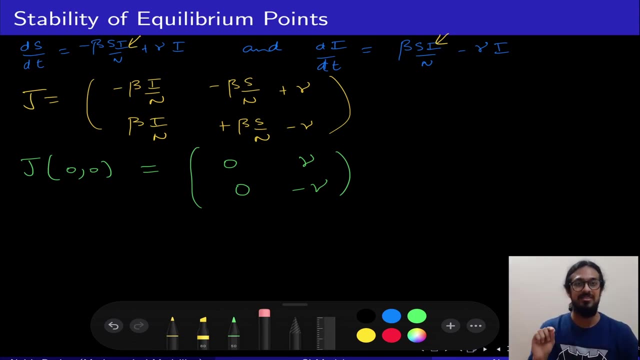 about those points now. the way we discuss stability is obviously as follows. if you are not aware of how to deal with stability, i have two videos on stability analysis. i'll link both of them right here and in the description box. you guys can check it out. i won't be explaining in detail about that aspect here. we'll just go into actually finding. 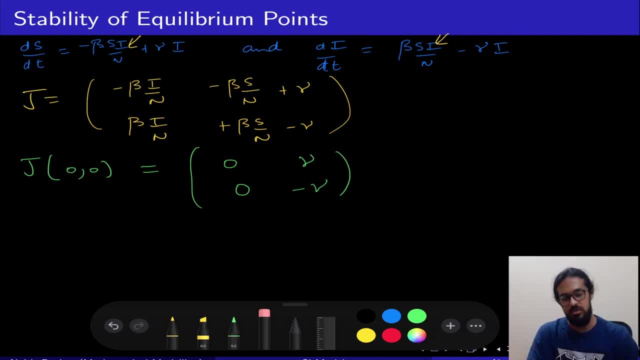 the stability. so we use the jacobian method. because our si model is a non-linear model. we can see that the s into i terms in both the ds by dt and the di by dt differential equations actually make it non-linear. so we find the jacobian. as you can see, i've already found it. 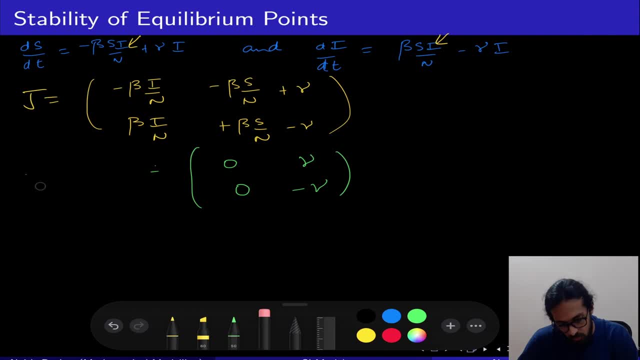 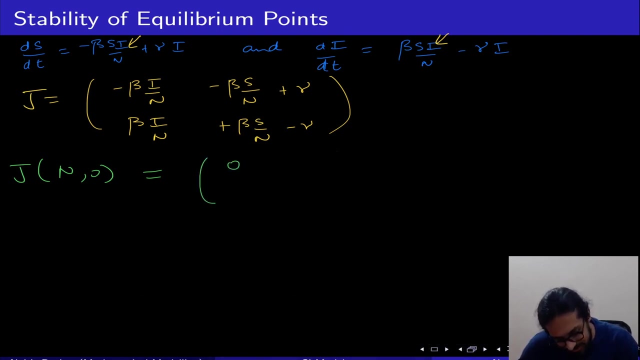 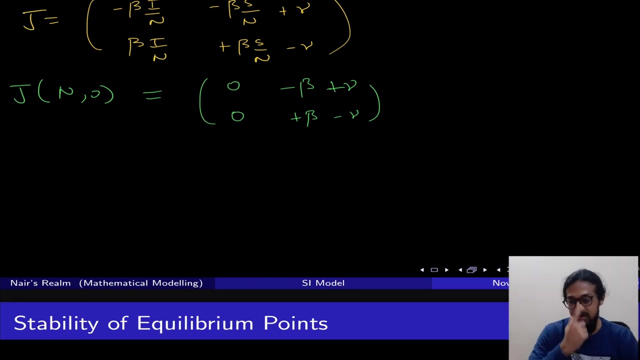 here and we actually try to find the equilibrium point first, at the disease free equilibrium point which is as follows: so i is zero, so the first term is zero, and here we have minus beta plus gamma, and here we have again zero and plus beta minus gamma. now the way we deal with uh, stability is uh, of course we try to find the eigenvalues of. 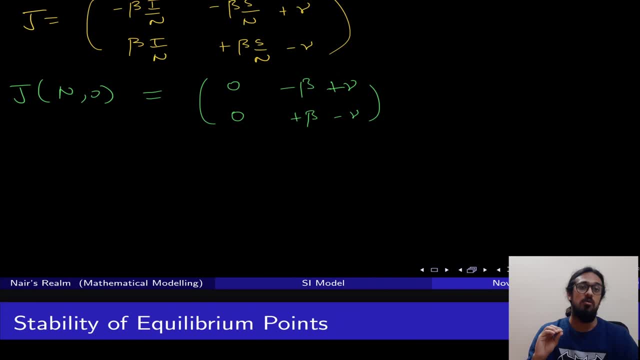 this jacobian matrix and try to see whether the eigenvalues are positive or negative or if they are complex. we have a particular method. again, i've explained those in the videos. you guys can check it out. so here i proceed to find the eigenvalues of this jacobian matrix, evaluated at: 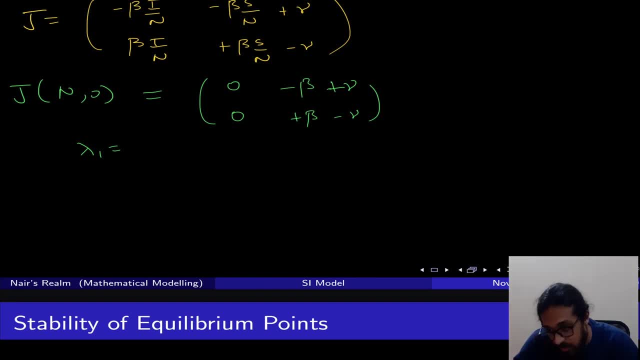 a disease-free equilibrium point and i get two eigenvalues. one is zero and the other is- sorry, beta minus beta minus gamma. so now this is a marginally stable equilibrium system because one eigenvalue is zero now the other eigenvalue can either be positive or negative. 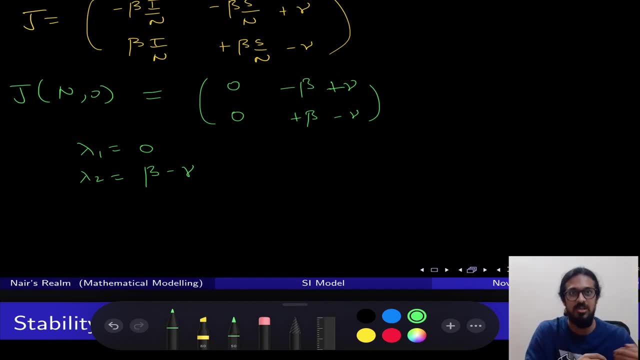 then we have a marginally stable system. if it is positive, we have an unstable system. so if this is less than zero- so that is beta is less than gamma- we have marginal stability. i will talk about what this uh, beta by gamma ratio represents, and it's a very important. 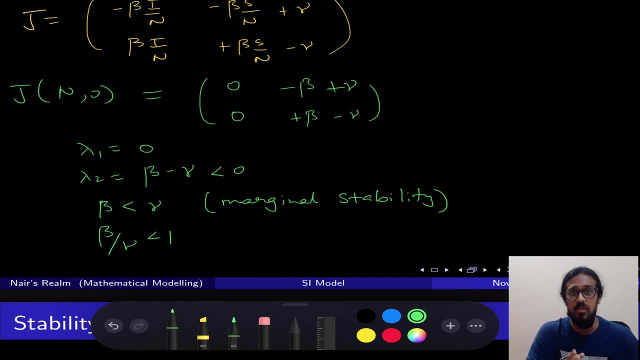 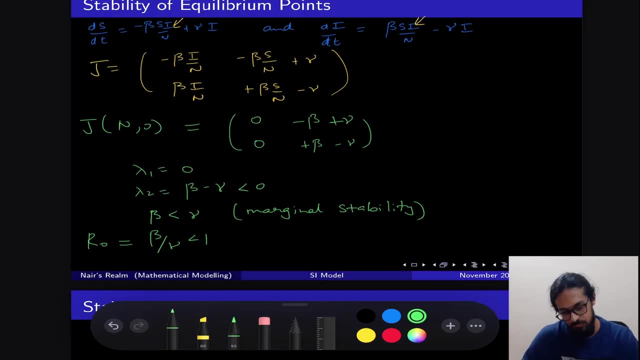 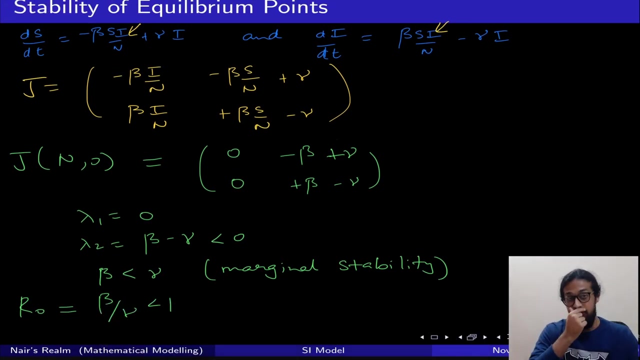 aspect of any mathematical model. it's called the r naught or the reproduction number. i will talk about it a bit more so now we have uh discussed the stability at the disease free equilibrium point. now we obviously want to talk about the stability at the endemic equilibrium point as well. 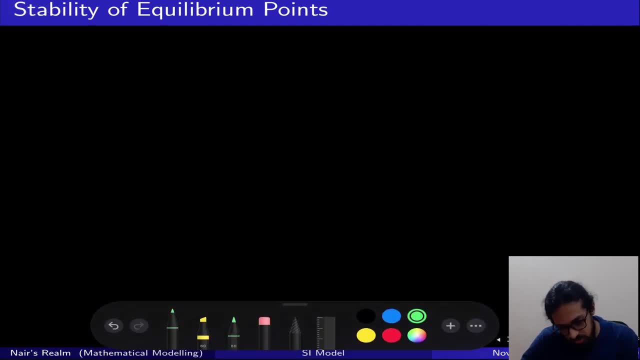 so if i were to evaluate the jacobian at the endemic equilibrium point, i would actually get the following matrix. you guys can solve it as well and verify that my math is correct here. so this is the jacobian matrix evaluated at the endemic equilibrium point. again, we find the eigenvalues for it. so 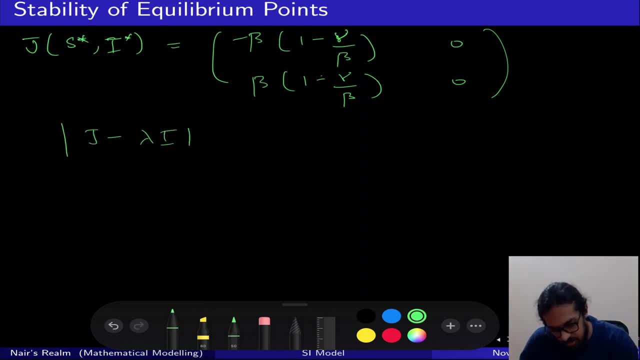 we do the determinant of j minus lambda i equal to 0, and we solve for lambda and we get lambda 1 equal to 0, lambda 2 equal to minus beta times 1 minus gamma by beta. now again, in this case we see that we have a marginal stability if the second eigenvalue is also negative, right. 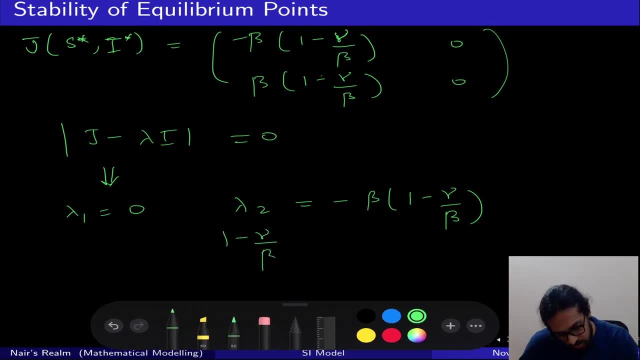 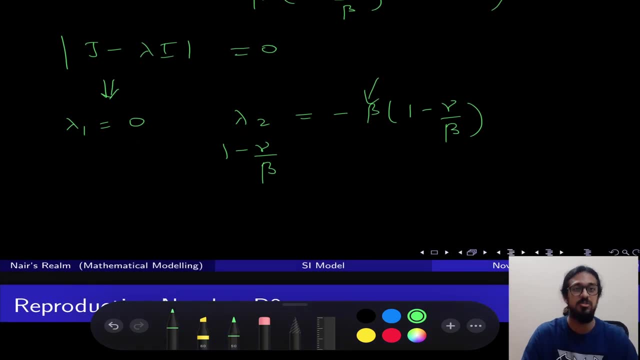 so that essentially means that if the first eigenvalue is negative, that means that the second eigenvalue is also negative, which means that that 1 minus gamma by beta, so beta by itself, is a positive value because it's a rate of transmission. you can't have a negative rate of transmission. worst case, the rate of transmission is 0 right. 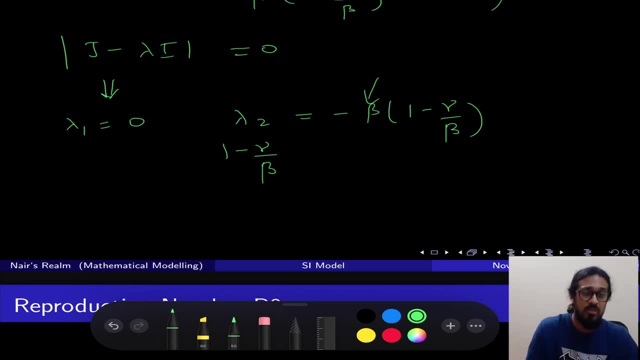 so it's always a non-negative number, so to speak. rate of transmission: 0 essentially means the disease doesn't exist, so you can think of it as a positive value. so that essentially means that minus beta is already negative. that means the other term, 1 minus gamma by beta, has to be positive. 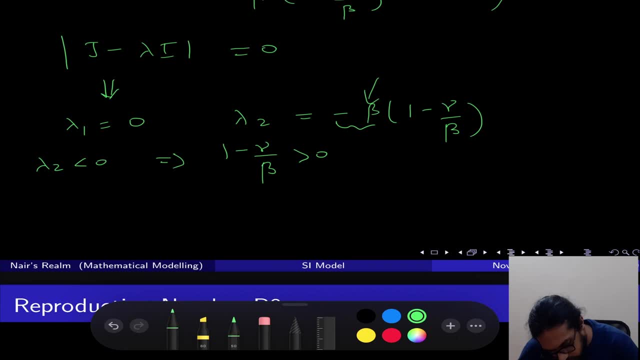 for lambda 2 to be negative. and we want lambda 2 to be negative because only if one of the eigenvalues is negative and while the other is 0, we have marginal stability. so this essentially means that 1 minus gamma by beta has to be greater than 0, and again this implies that gamma by beta 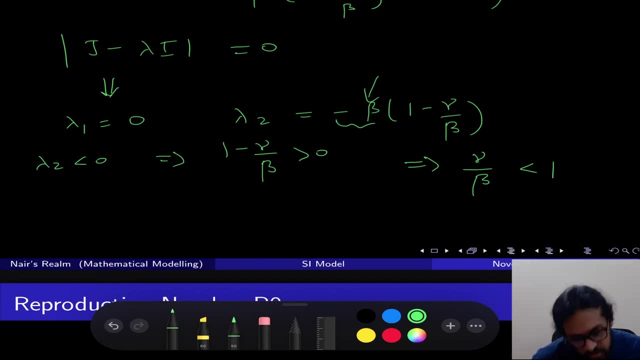 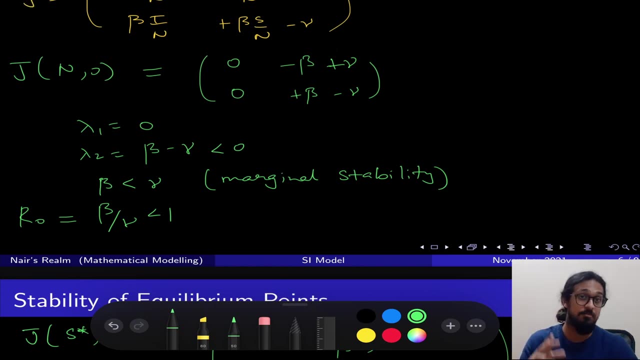 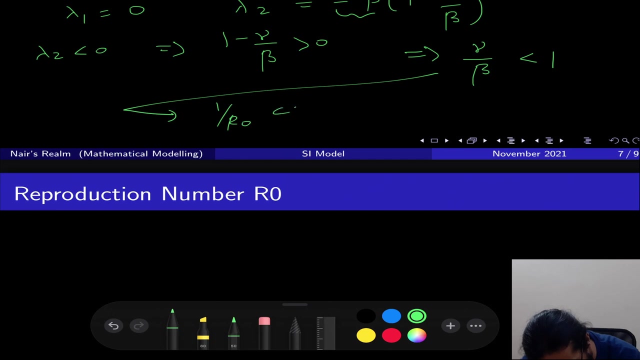 has to be less than yeah, gamma by beta has to be less than 1. so now from the previous slide we can see that r naught is defined as beta by gamma. so if i were to plug that in here i would see that 1 by r naught is less than 1, or this implies r naught is greater than 1. now that concludes. 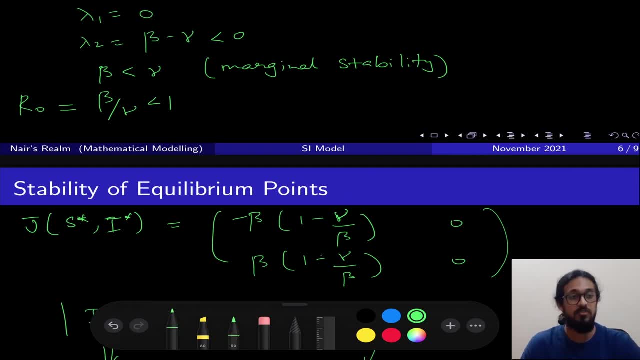 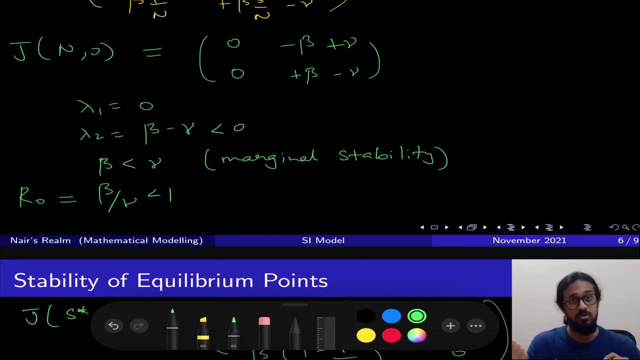 our analysis of the stability of the system of the equilibrium points. now we talked about the equilibrium at two points. one is the disease free equilibrium and the endemic equilibrium. both of them came up at the end of it. we both ended this condition on this value called r naught. so what is r naught? it is actually the reproduction number. 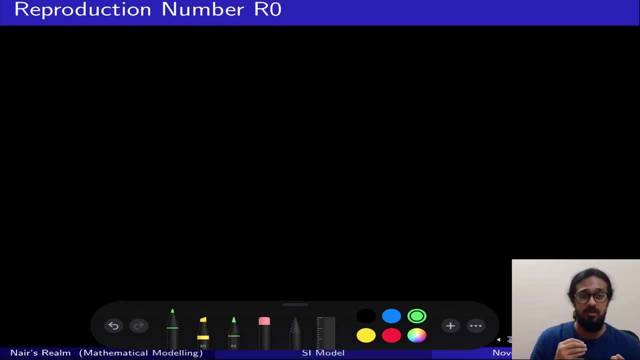 so the reproduction number of any disease can be thought of in the following way: if i have an individual, if an infected individual, how many other people is he going to infect? right? so i'm infected with uh, the common cold. if i'm infecting one other person, 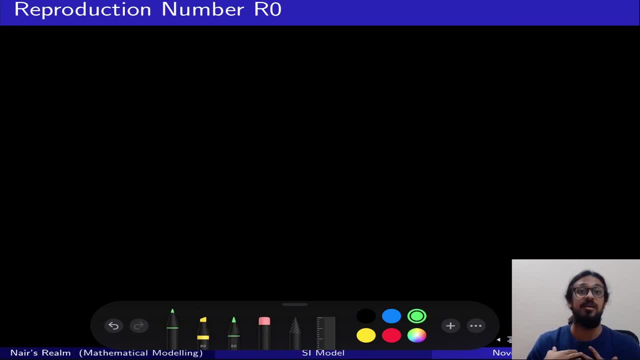 then the r naught of that disease is one. if i'm infecting two people, then the r naught is two. now, obviously, i'm just one infected individual. there may be hundreds and thousands of infected individuals. so we average out all those values and we come up with an r naught, so to speak. 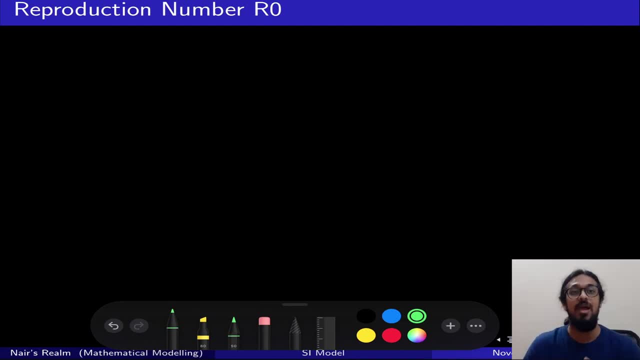 now, if you think about it, if an r naught is greater than one right, if i am infecting more than one person, or even one person or more than one person, then essentially it means that the disease is spreading and the higher the r naught value. 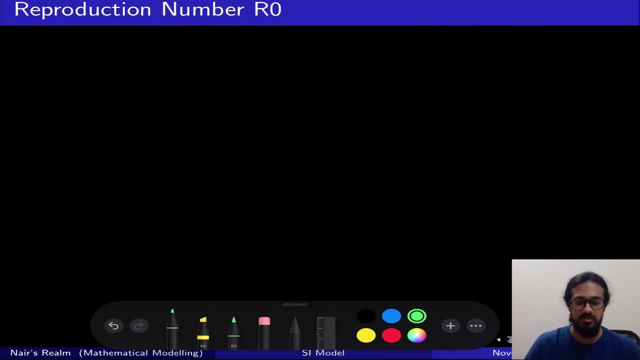 the more rapidly or the more exponentially the disease is spreading. so r naught, which is in this case beta by gamma, dictates whether the disease is on the tapering end. now think of it this way: if r naught is less than one, that means i am infecting less than one. 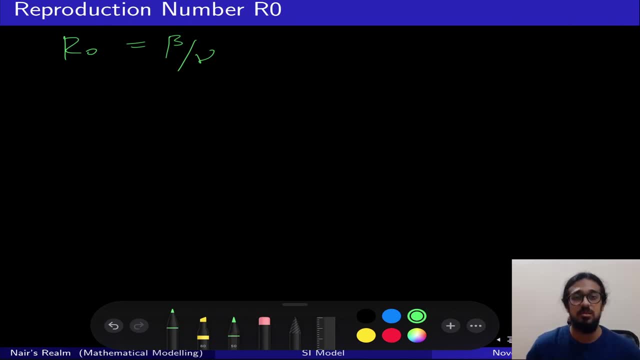 person. it essentially means that the disease isn't able to transmit or transfer between people. so that means that the disease is reaching towards an endemic uh state where in only some regions where the r naught value is higher there could be some outbreaks of infection. but overall,